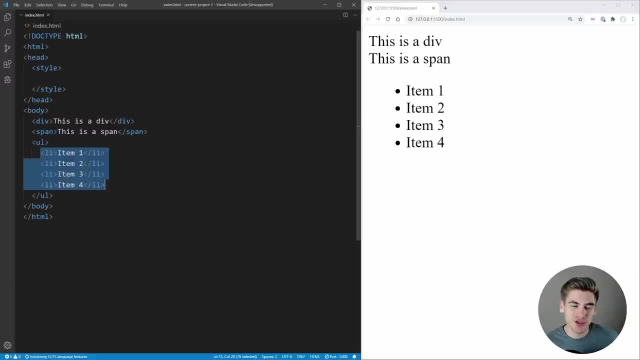 Now to get started. I have a really simple HTML page. We got a div, a span, a ul with some li's and cypher, And from here I'm going to show you all the CSS selectors you need to know in order to properly style all of these different elements. 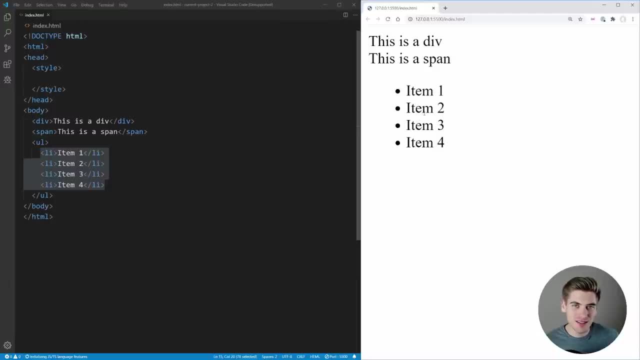 And to get started, I want to go over the most basic types of CSS selectors which you're going to see everywhere, And the very first CSS selector I want to talk about is going to be the universal selector. This is the asterisk symbol, this star here and what this? 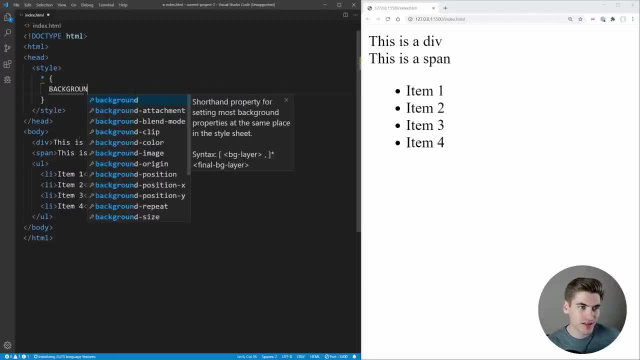 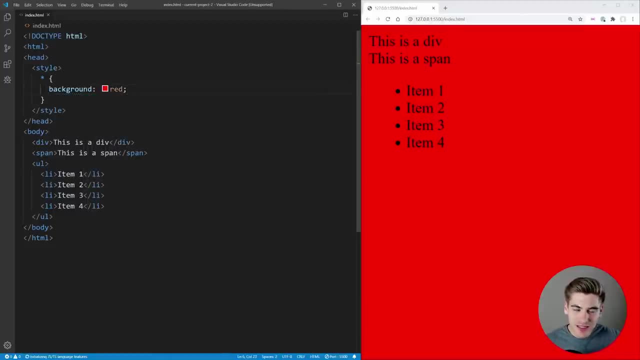 says is to select literally everything. So if I say oops, background is going to be red. this is going to change the background of every single element: Our body, our div, our span, our ul, our li, Every single element is going to have a background color of red because this star asterisk symbol is. 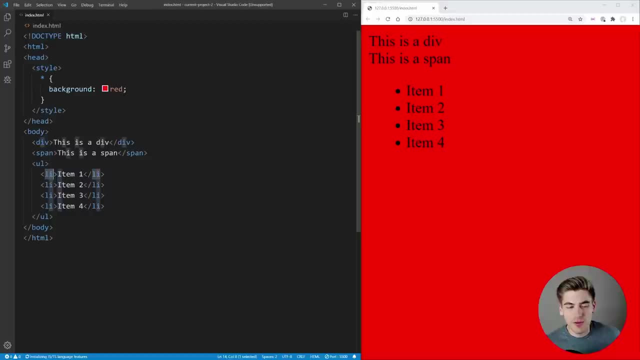 selecting every single element on our page. If we want to only select certain elements, though, we can use the type selector, which is going to be for selecting element types. So we could say, for example, div- we just type out the element and now our divs are red. We could say li and. 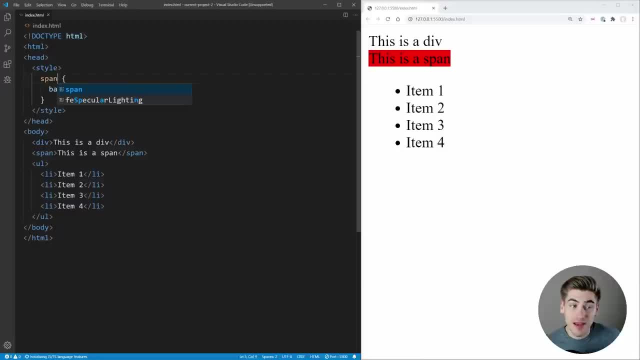 now all of our li's are going to be red Or span, and now our spans are going to be red. So we can select individual elements based on the actual type that the element has, based on that tag that we specify in the HTML. Now the next type that we can use is a class selector. 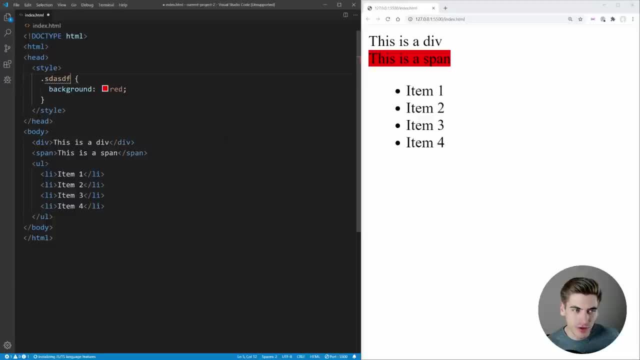 So a class selector works by: you put a period and then you type in whatever you want and that's going to be your class name. So we could say, for example, red is going to be our class name And if we save, you'll notice nothing is red, and that's because you need to apply classes. 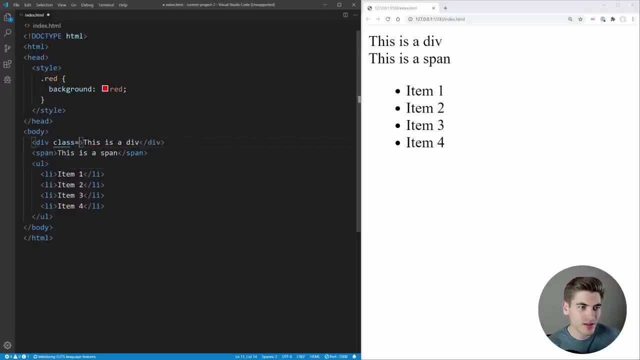 to your HTML. So I can come down here and say that our class is going to be equal to red and our div is red. Let's say I want this item to be red. I can give it a class as red as well, and now that item is red also. So any element that we give the class of red to is going to have this style. 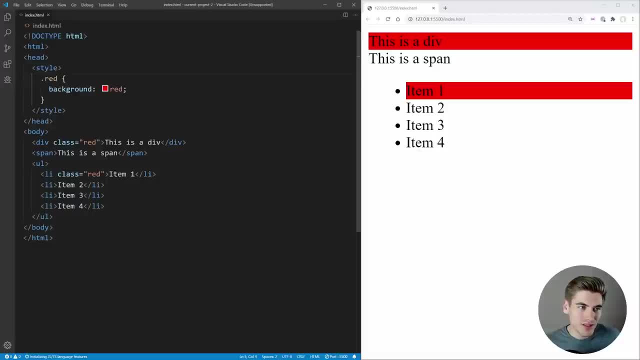 here because we give it this dot red selector. So anytime you want to select a class it has to start with dot and then the class name. Another type of selector is going to be the id selector. It's very similar to the class selector, but you start with the pound sign and then you type in. 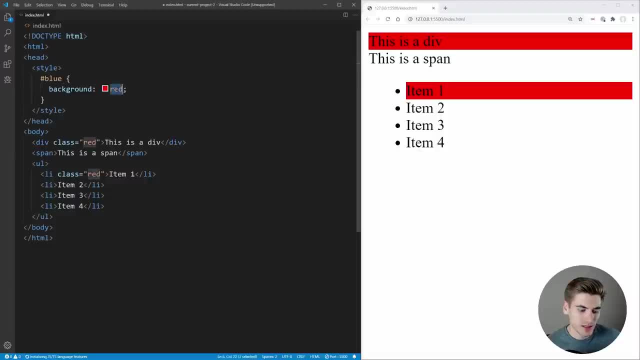 the id that you want it to be. So let's say, for example, blue is going to be our and we'll change this color to blue here. Let's give this span an id of blue, So we just say id equals blue, and now we save and you can see our span has that blue background color. 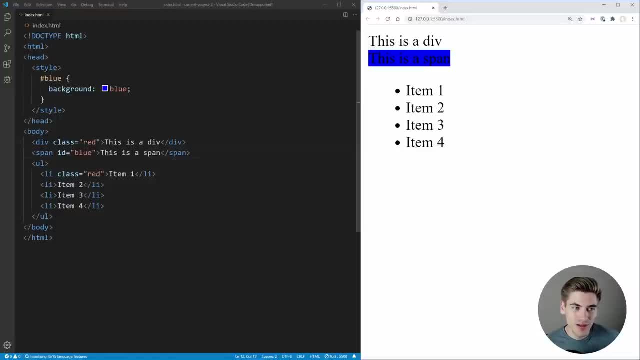 But one important thing to note is that if you use id selectors, you can only have one id on a page, So an id selector is generally something you don't want to use because you're going to only have one on a page. It's very specific and it's generally not too useful. Also, when you're using 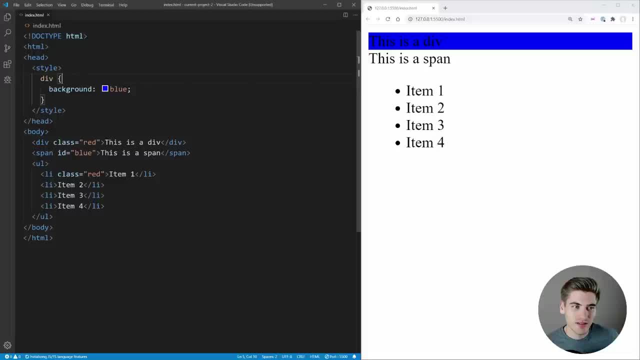 a selector like div, for example. this is also not very useful because I don't probably want to style all of my divs exactly the same. I probably want to style some divs differently, some not the same. so you're generally not going to use the element selector Most commonly out of these selectors. 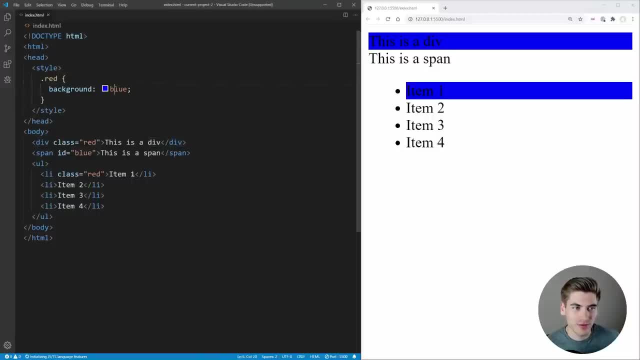 you're going to use that class selector where you're saying red, for example. This is because you can share this across whatever elements you want by just giving them a class. You can share it between multiple elements. you can have it on just one, you could have it on ten. 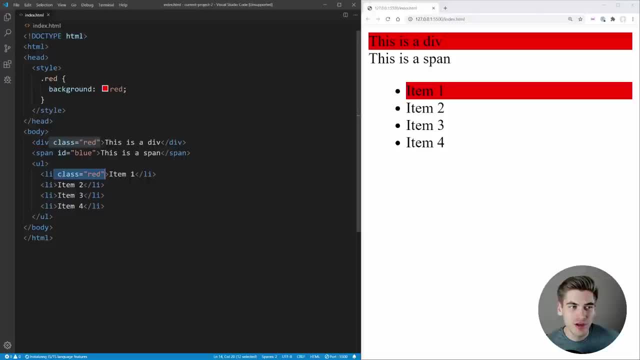 you could have it on none. It's really flexible and that's why, generally, you're going to use class over ids and elements. Now, this is the most basic types of selectors, but what happens if you want to combine together different selectors? Well, that's actually really easy to do. What if I 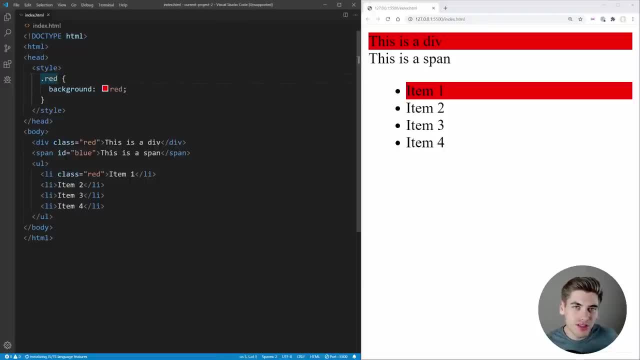 want to select only divs that have the class of red, Well, all you need to do is put these selectors together without any spaces between them, So I could just say div dot red and I save, and now you can see: only divs that also have the class of red are going to have this background. 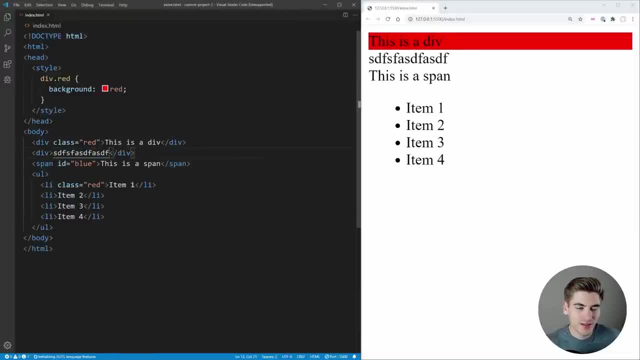 color of red, Because if I add another div with some random text in it, you can see that this is also a div, but it doesn't have the red background because it doesn't also have the class of red. So that's something really important to know. if you want to combine together selectors, you just 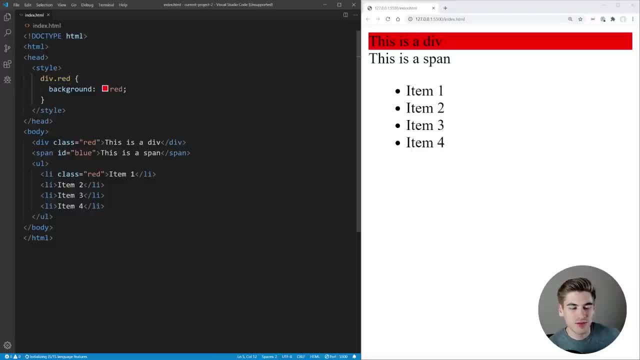 keep adding them together without any spaces. For example, I could say divs that have the class of red and the class of green text, and if I give this a class of green text and I give it a color here of green, you can see that now only divs that have the class red and the class green text. 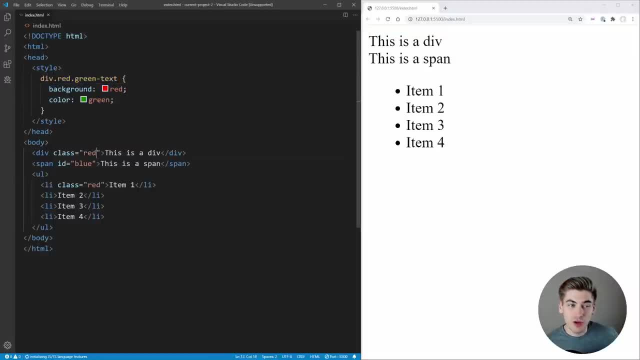 have these styles applied. If I remove the green text class, it no longer matches all of these selectors, so it's no longer going to have those styles applied. Now, what happens, though? if I wanted to do like an or type of scenario, Let's say, let's just remove all this. I wanted to select. 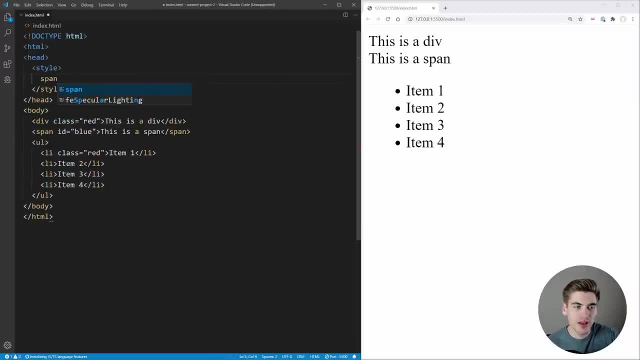 all of my spans and I wanted to give them a certain style. and I wanted to select all of my li's and also give them the same style. Well, all you need to do is put a comma between your different selectors, and now it's going to select both of these things. We could say our 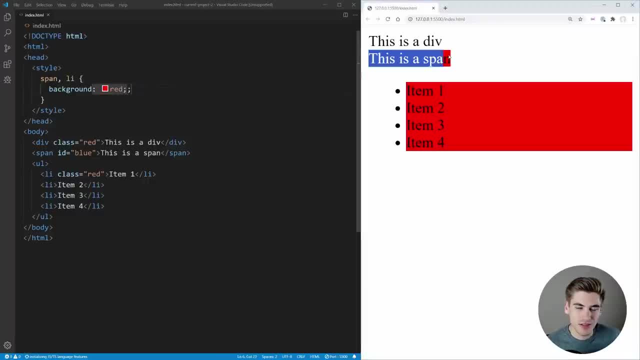 background is going to be red and now you can see our span has a background color of red and every single one of our li's also has a background color of red, and that's because we put the comma between them. and we could even go a step further and go that any span now is red and 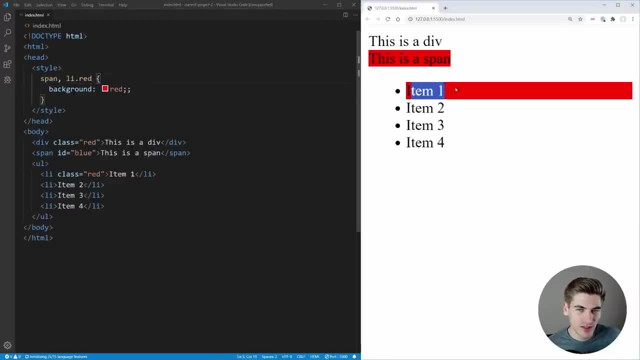 any li with the class of red is also red, and we save, and you'll see, only this first one which has the class of red is red, and our span is red as well. So we're able to combine together all of these different selectors, whether it's with commas or by just concatenating them together. 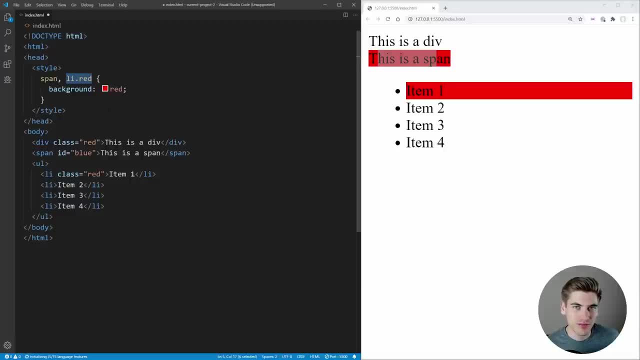 in order to do and operations as well as or operations. So that right there, just those few little selectors, is probably about 40 percent of all the css selectors you're going to write, because generally you're just going to be selecting things based on classes combining. 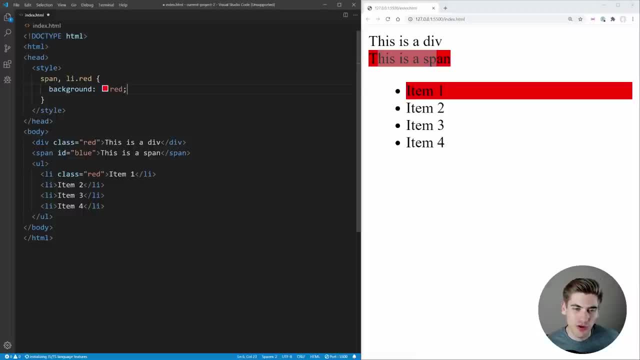 together classes or using the comma to say this class or that class. But what if you need to do something a little bit more nuanced? What if you want to select elements inside of other elements? Well, there's actually a really easy way to do that. Let's say that we want to get all of the li's. 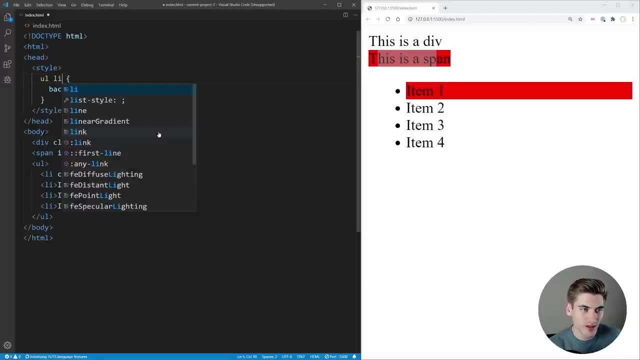 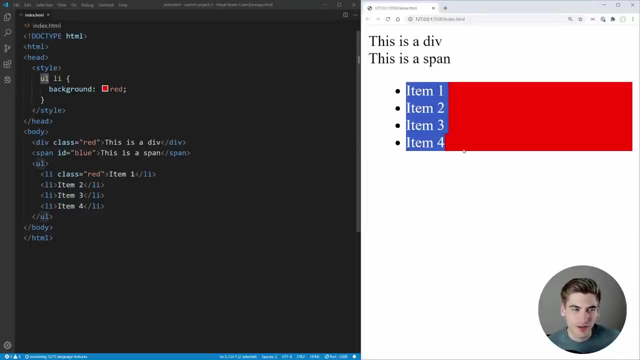 inside of a ul. We could say ul, space, li and save, and now you can see all of our li's are having this background color. So a space essentially says that anything inside of an element that comes before it, So any li inside of a ul is going to have this red style here and let's just change our mock-up here a. 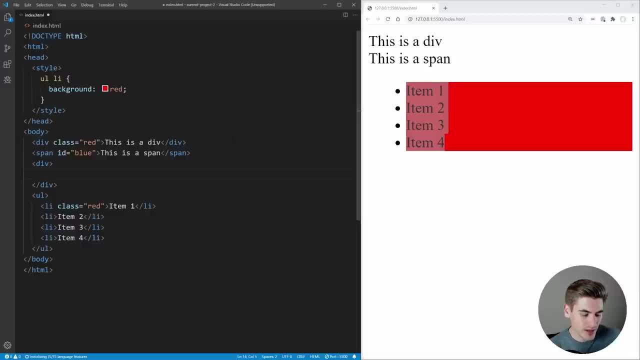 little bit. We have a div and let's say inside of that div we're going to have a span. and then inside of that span we're going to have b and we're just going to say nested text, Just like that. and now let's say that we want to select any b tag that's inside of a div. Well, we 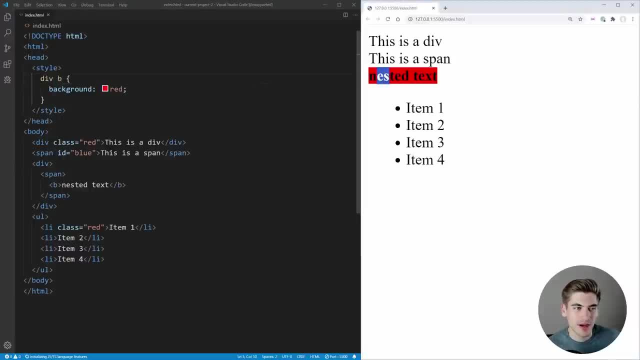 could just say div and b, and now you can see this has a background color of red because this space selector essentially says anything inside of a div. whether it's the direct child, a child of a child, a child of a child of a child of a child, it doesn't matter, as long as it's inside of a div. 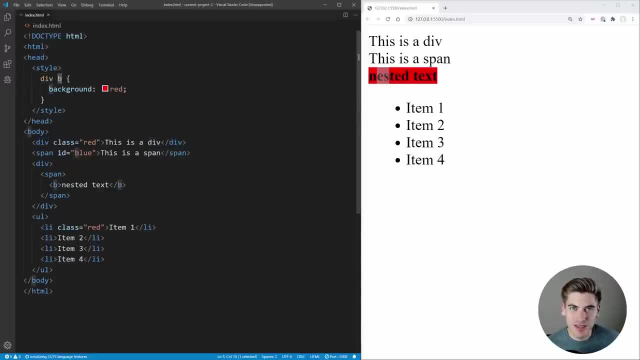 That's all that matters and that it's also matching the selector of the b tag. And again, you can say dot red, for example, and now any dot red class inside of a div is going to have this background color of red. You can use any different combinations of selectors you want. I'm just 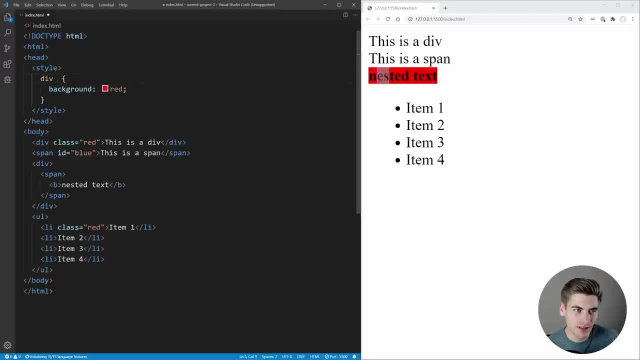 generally going to use element selectors because it's easier to get the point across. Now, another type of child selector that you can think of is the direct child selector, and this one is using the greater than symbol here, and then, if we put b, for example, on save, you're going to notice our 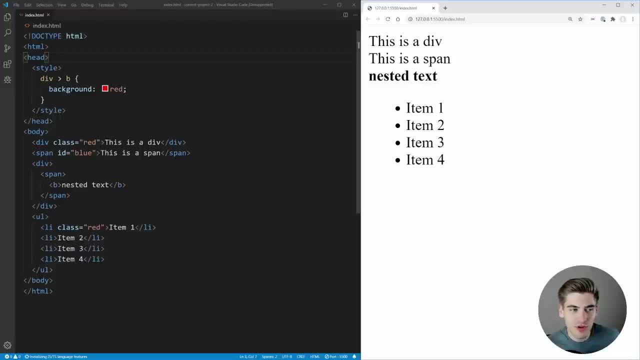 b tag no longer has that red color and the reason for that is because this b tag is not direct child of our div. This says it has to be the direct child and our direct child is actually this span here. so the b is not our direct child, our span is the direct child of our div. If we 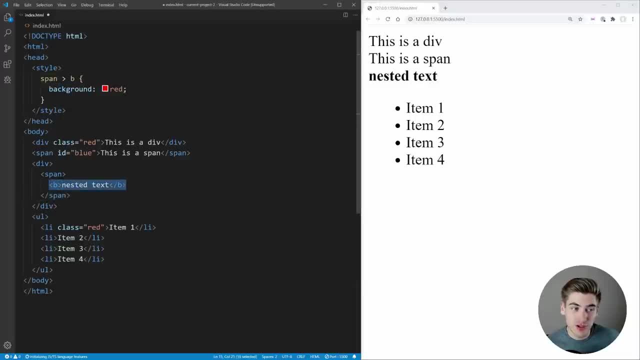 change this to be span, then b- you can see the b tag- is the direct child of our span, so this will properly give it this red background color. So this greater than symbol is always going to be direct child, while if it's just a single space it can be any level of child it does not have. 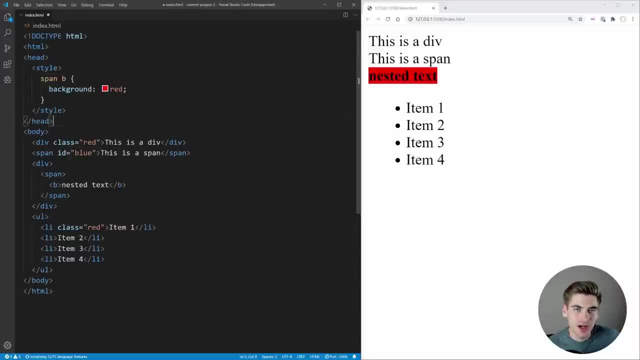 to be the direct child. Now, the last two selectors that I want to talk about in this section are going to be based on sibling selectors, so it's essentially getting a sibling of an element, and the way you define a sibling is inside of this html. we have our body. 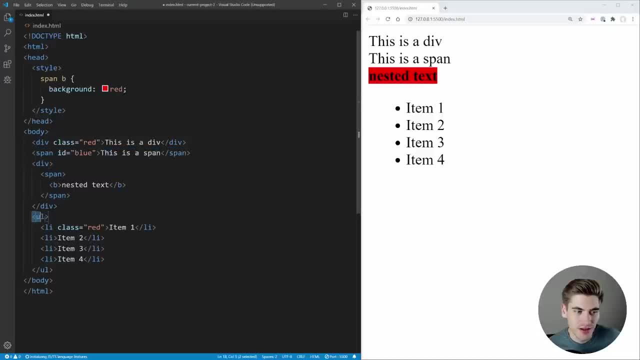 and each one of these elements- our div, our span, this div and this ul- are all siblings in the body. and then these lis are all siblings in themselves because they're all inside the same element, at the same level of nesting. that's how you define a sibling. so let's say that we wanted to select. 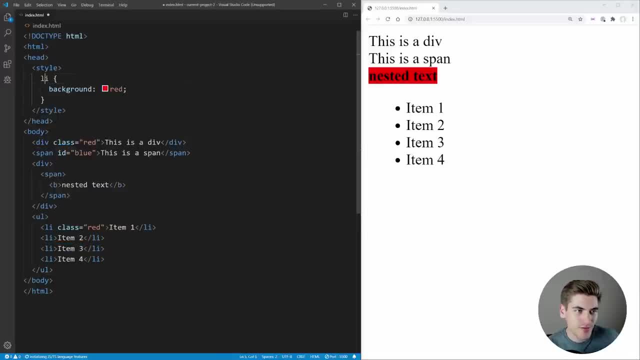 every single, let's say, li that comes after an li with the class of red, so we can say lired. and then if we put a tilde symbol, this is saying: give me every single li that comes after an li with the class of red. and if we save, 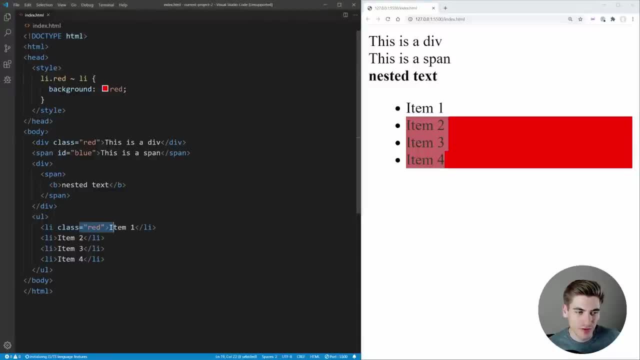 you can see all three of these lis come after this li with the class of red. if we actually move this class red down to item two and save, you'll notice that even though item one is a sibling of item two, it doesn't actually get selected by this selector because it only selects elements. 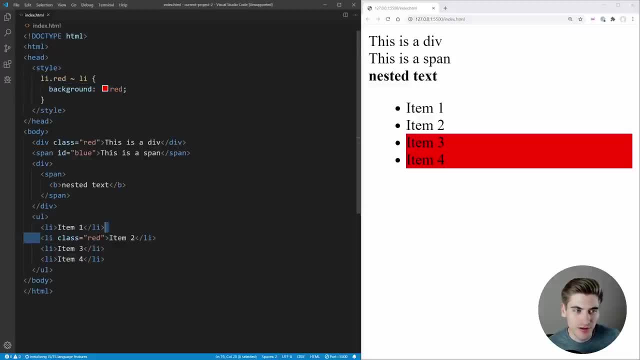 after. so we found the li with the class red. it's right, here now we're only getting the siblings that come after, which are items three and four. but what if you only want to get one sibling? you don't want to get every sibling, you only want to get the direct. 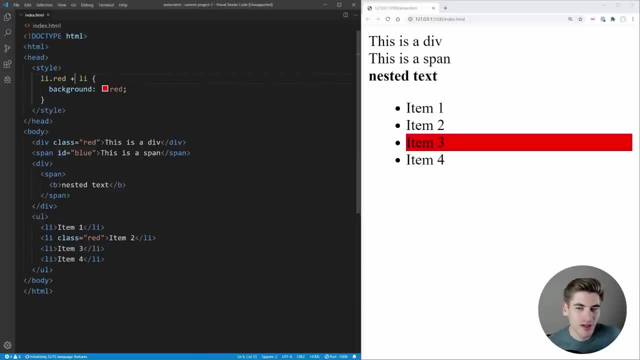 sibling. what you can use instead here is the plus symbol. and now, if we save, you'll notice that this will only get the very next child that is going to be having that li here. and that's because, unlike the general sibling selector, which is the tilde that selects all, 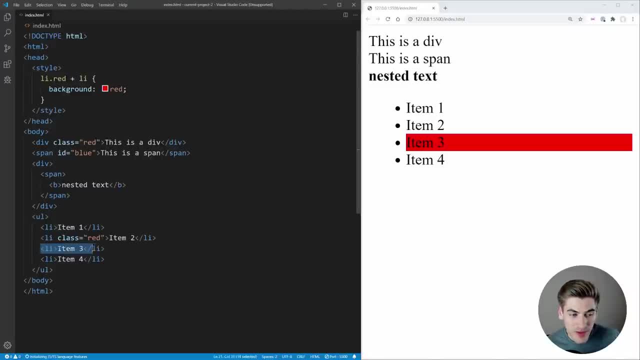 that are afterwards, the plus is only going to match the very next element that comes after it. so we're only getting the li that comes directly after this li with the class of red. and if we were for some reason to say that this has a class of green and we wanted to get li's that have the 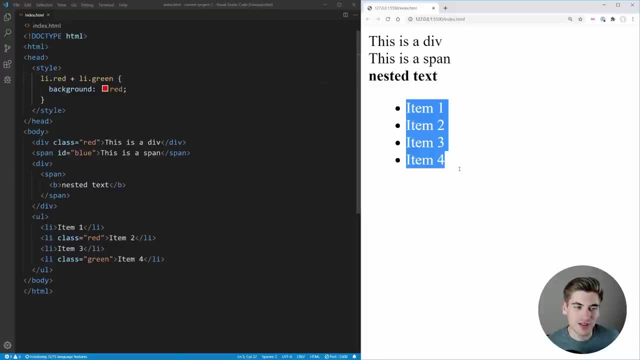 class of green and we say, if you'll notice, nothing is actually styled. and that's because this plus symbol only checks the element directly after which is item three, which does not have a class of green. so it does not actually match this selector. now, with these different types of 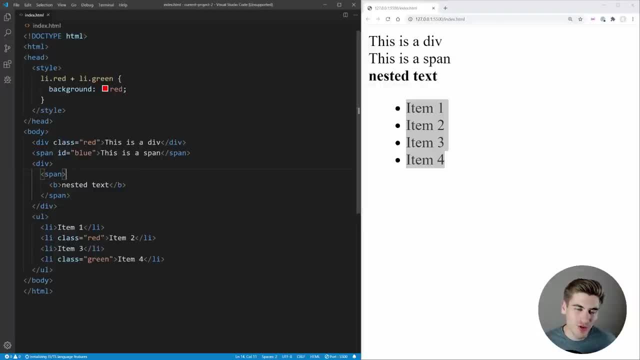 descendant and sibling selectors. that's probably another 20 of all the css you're going to write. and next i want to talk about pseudo classes, which are probably again another 20 of all your css styles, because they're really important with css and pseudo classes are essentially ways to style. 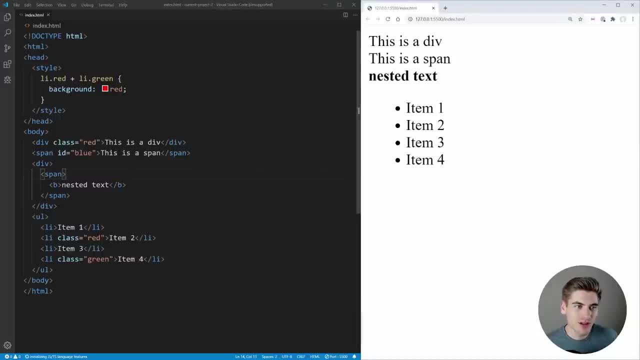 elements based on how a user interacts with the page. so let's, for example, say that we want to select every single li that a user hovers over. what we do is we put this colon and then type in: hover. every single pseudo class is going to have. 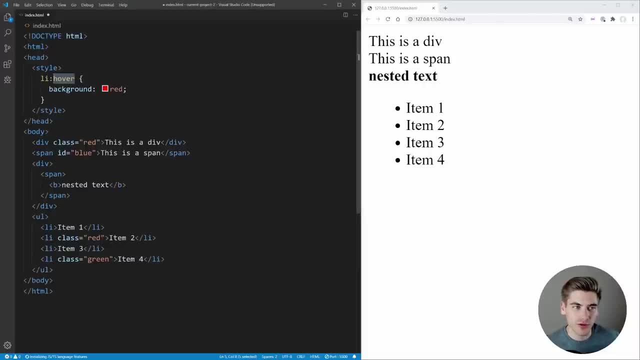 a colon followed by the actual thing that we want to check for, in our case hover. so now, if we save and we hover item one, two, three or four, every single one is going to have that red background as soon as we hover over it. another type of pseudo selector is the focus pseudo selector. 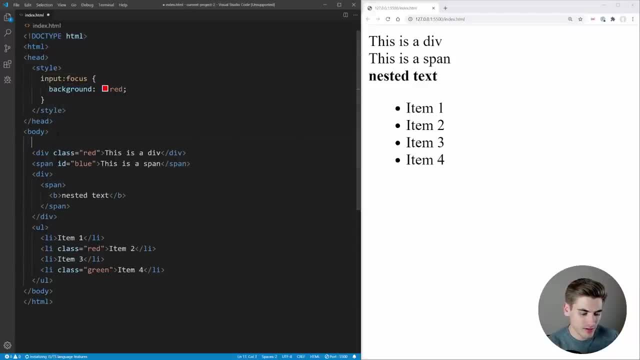 so let's get an input element inside of here. let's just say we're gonna have an input and if, as soon as we click inside this input, we're essentially giving focus to this input, we're focusing on this element by clicking on it. so now it has that background color of red and when we click outside of it you can see it. no, 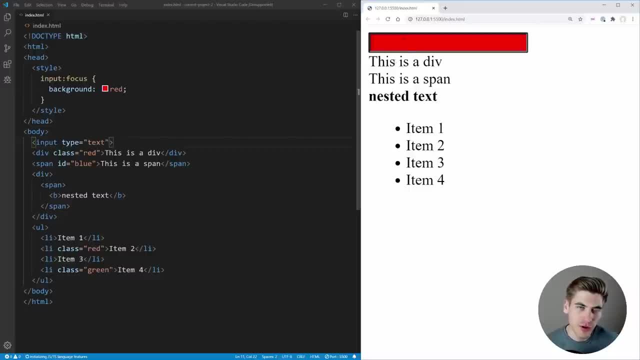 longer has that background color, so this is based on where the user's focus currently is on the page. this works with things like buttons and form inputs, which is where you're mostly going to see this. speaking of input selectors, we can come in here and let's just change this to the required. 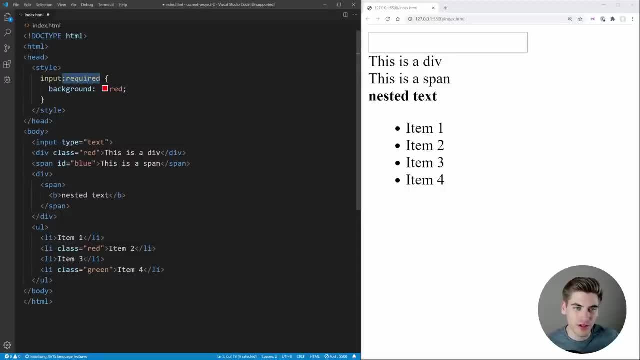 selector. this is only going to select inputs that have the required attribute. so if we come in here and say required now you can see our text has a red background color, while if we do not have required, it just has a normal white background color. also, we can check check boxes by saying checked. so if we were to come in here and say that this is a check box instead, 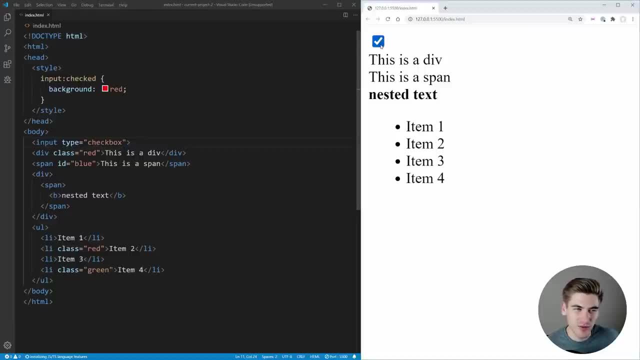 whenever we check this check box, the background color should be red. but since you can't really modify the background color of a check box, i'm going to come in here and change the margin to be 50 pixels when it's checked. so if we click this, you'll see it has a bunch of margin around it when it's checked. 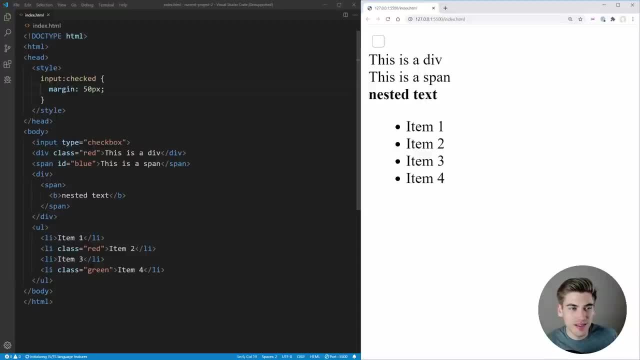 and when we uncheck, you can see all of that margin disappears. and again, just like with checked, we can check for disabled and now if we save, you'll see nothing happens. but if we change this to be disabled and save, you now see we get that margin around it. 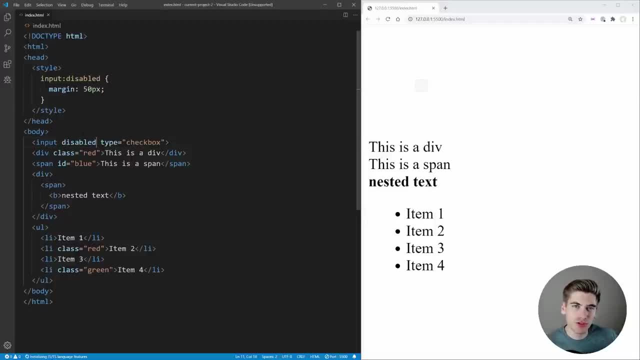 because it has that disabled status applied to it. now, those are the most useful selectors when it comes to interactivity with the page, whether it's disabled, hovered, focused, all that fun stuff. but there's also another whole class of pseudo classes, which have to do with where elements are positioned. 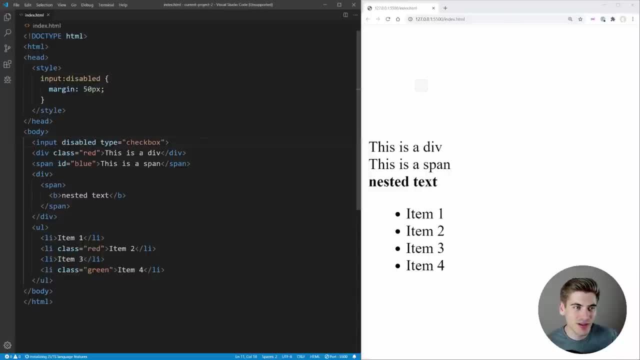 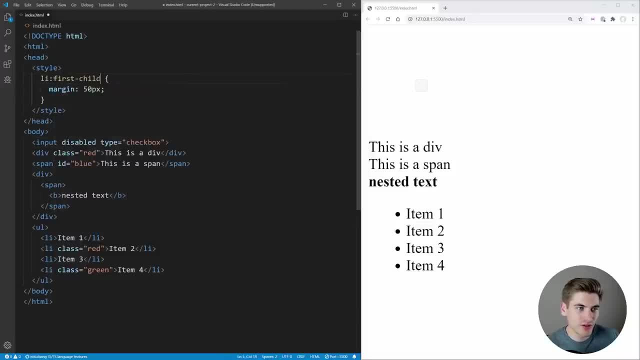 by selecting our li's, we can say li, first child and we want to come in here and just say background is going to be red and if we save, you can see the first li child has a background color of red and the reason that this is working is it's the first child inside of the parent in our 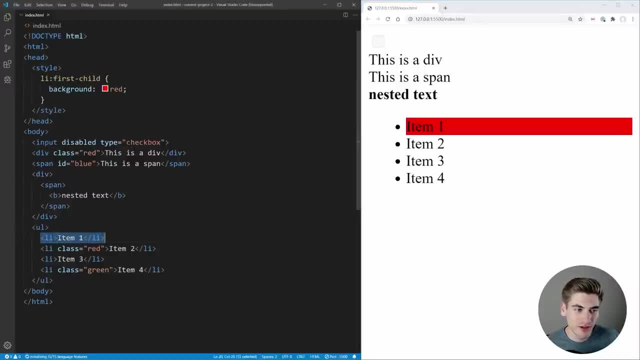 case, our parent is the ul and this li is the first child. let's just come in here and say what if we wanted to select the first li with the class of red? well, now you'll notice this no longer works, because first child only selects the very first child, which is item. 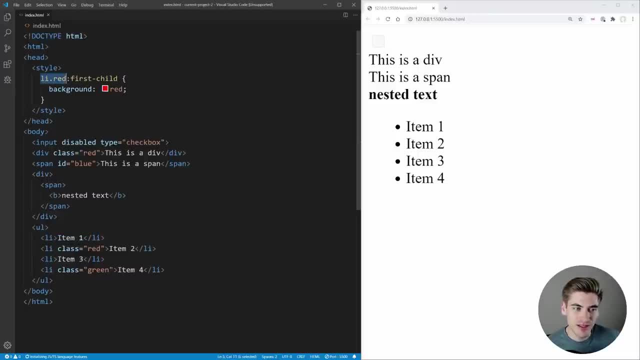 one. it doesn't select the first child that matches this selector, it just selects the very first child. we can do a similar thing to first child where if we just get rid of this red here, you can see we have the first child selected. we can come in here and say: last child, that's going. 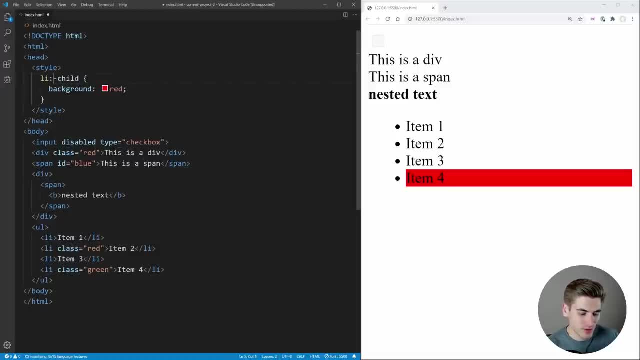 to select the last child for us and then, if we want to select some combination in between, we can say nth child, and in here you just pass the number, for example three, or you can pass a number, like a formula, that has n in it, so we can say 2n. this is going to select every other element. 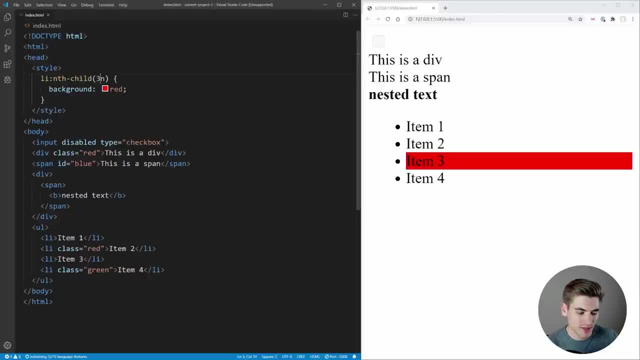 you can do 3n and it's going to select every third element. element. we could say: you know one or not one, two, n minus one. that's going to select every other element, but it's going to offset by negative one, so it's going to start with one instead of two. 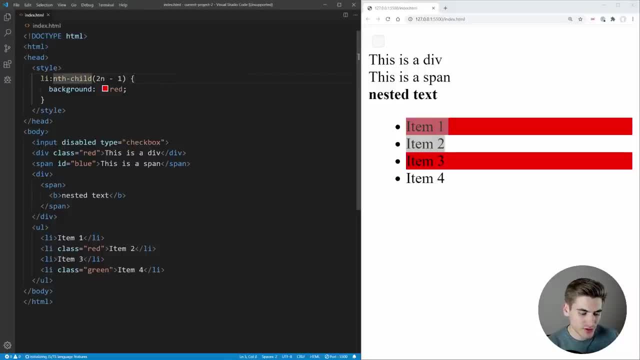 and so on, so you can write in any formula you want. you can also do the same with last whoops and last child, and it does the same thing, but it starts from the bottom and goes up, and then, lastly, there is something called only child, which just is like this: and it's going to select if it's the 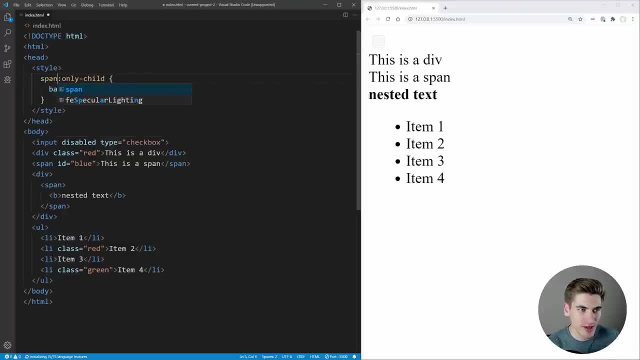 only child. so we can say that we want to select any span that is the only child. and you can see that this span here is the only child inside of this div, so that's why it has the background color of red, while this span is next to a bunch of other children, so it does not have that red background. 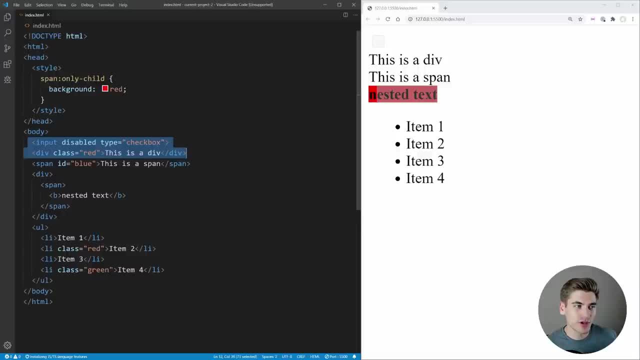 color and very similar to the child. we have something called type. so we could say here: first of whoops of type, and now you can see that the first element of this type span is the only child. so we can say that this span is the only child inside of this div. 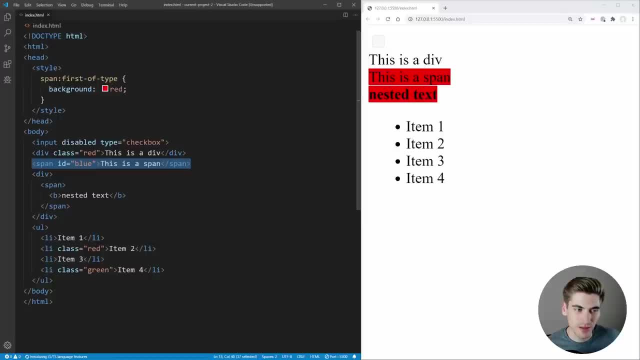 that you find inside of our selector. so our very first span element here and our first span element in this container both have a background color of red. we could also do last of type and if we change this to li, for example, you'll see the last of an li in our list is going to have that. 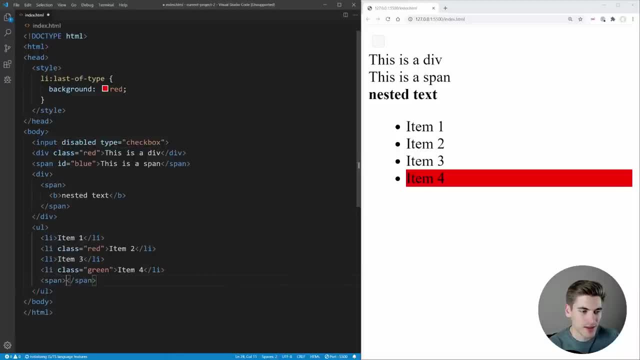 selector. if we came in here and added, for example, something else like a span inside of here and saved, you can see that this li here at the bottom still has the correct styling applied to it. even though it's not the last element, it is the last of the type li, so we can say that this is the 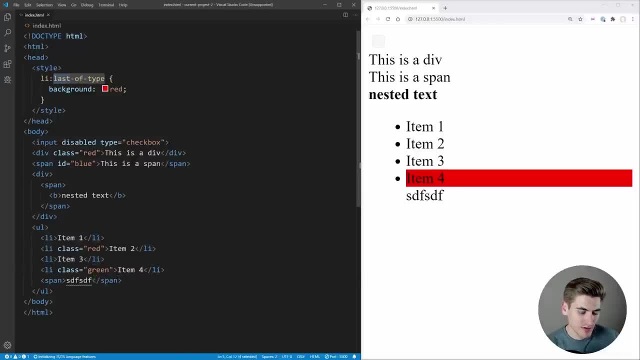 last of type, which is what this of type stuff is doing. we also have nth of type- same exact thing. we could say two, or you can say nth last of type. it's all going to work exactly the same. and then finally you have only of type. like this: get rid of the two here. this is going to return if it's. 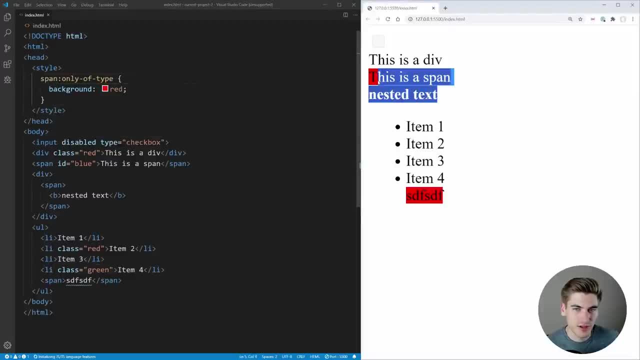 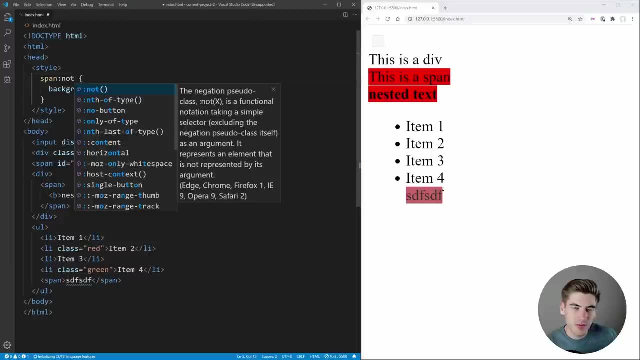 the only of that type. so if we did span again, you can see that these are the only spans in their containers. now, the very last pseudo class i want to talk about is the not pseudo class, and this, in my opinion, is the most important one, because it's the only of that type. so if we did span again, 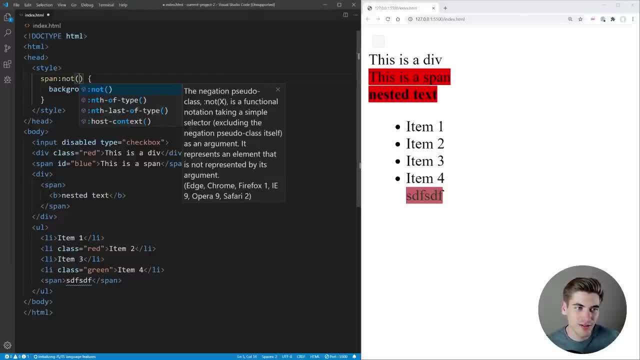 we could see that this is the only of that type. so if we did span again, we could see that this is powerful because you can pass it any other selector you want inside of here and it's going to essentially say: i want to select any element that does not match the selector you pass to it. 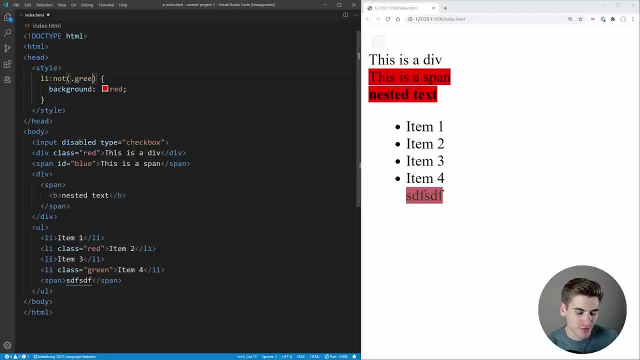 so let's say we want to get any li that does not have the class of green. now you can see we get item one, two and three, but since item four has a class of green, it is not being selected by this selector because of this- not pseudo- class. now we've covered pretty much all the pseudo classes. 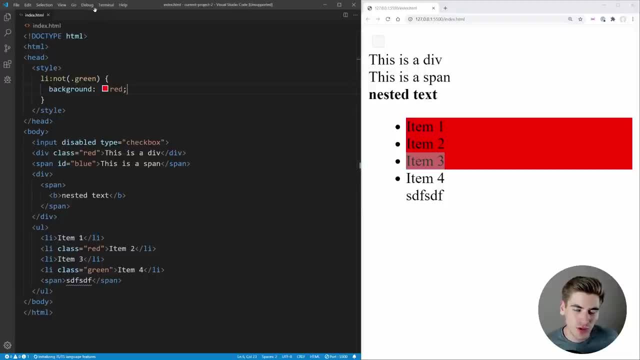 that you're going to need to know and we can move on to pseudo elements which are much simpler you need to know about. let's come in here and say that we're going to select our div here with the class of red and we want to get the before pseudo element. so it's going to be two colons followed by 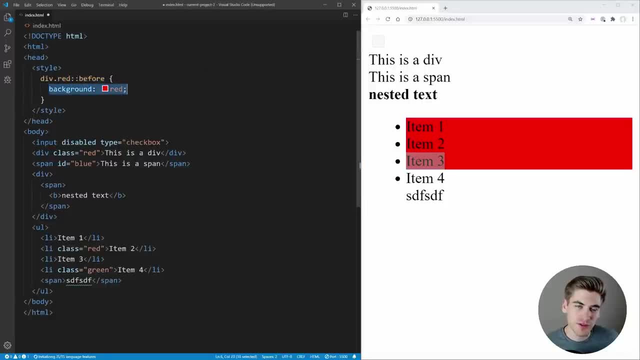 the pseudo element which in our case is before. and if you're confused about pseudo elements, i have a whole video on them in the cards and description. i'll link for you. but in here let's just put a content which is just going to say before, and then we'll do a background. 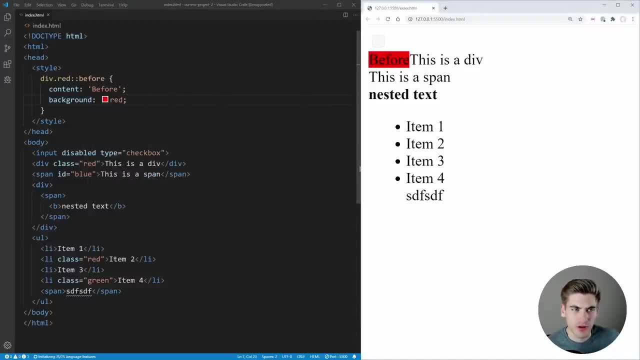 of red and, as you can see, the text before is being appended before our div with the background of red and the other pseudo class here, pseudo element, i'm sorry- is after. so let's just change our text after and you can see that shows up after our div, fairly self-explanatory. and again, if you 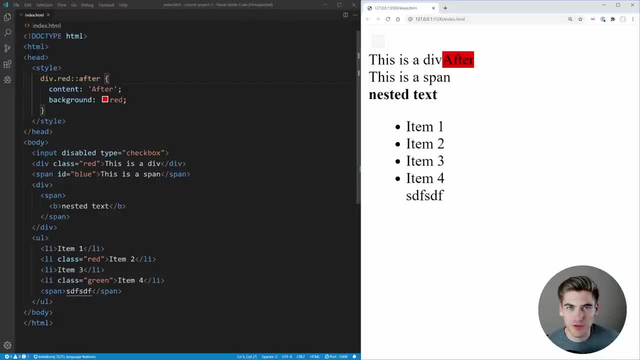 want to check these out. i have a full video on them where you can really learn all about the use cases and how you can use pseudo elements. now, the last set of selectors i want to talk about this whole video are attribute selectors, and these probably cover about the other five percent or 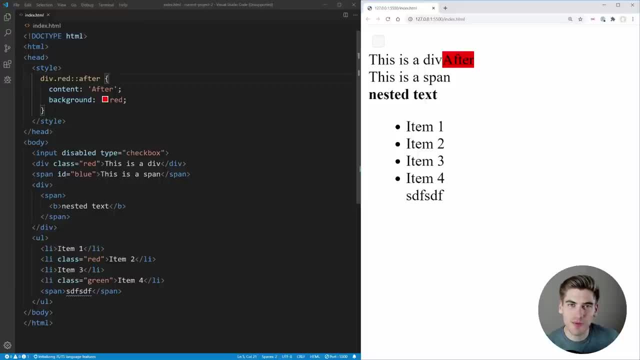 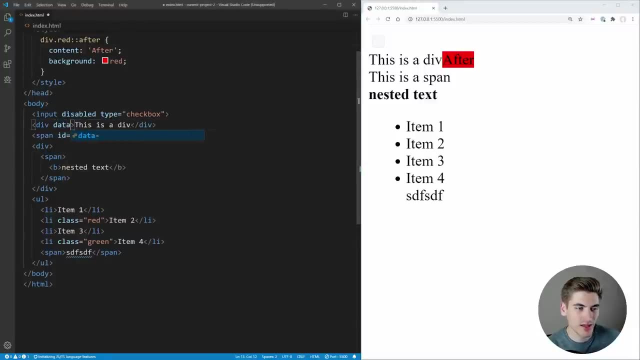 so of your css selectors. they're much less common, but they're pretty powerful and have some really great use cases. so let's say i come down here on this div, instead of having a class of red, i give it a class of, you know, data red. this is a data attribute, custom one that we applied to. 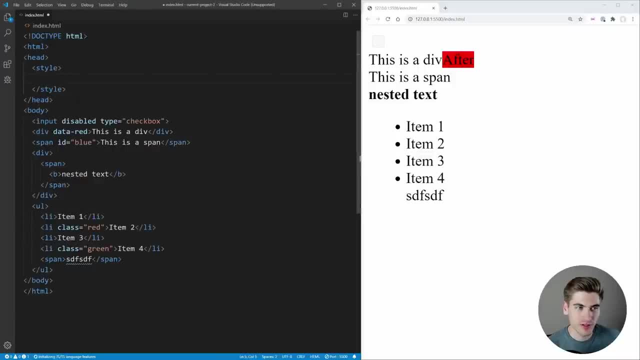 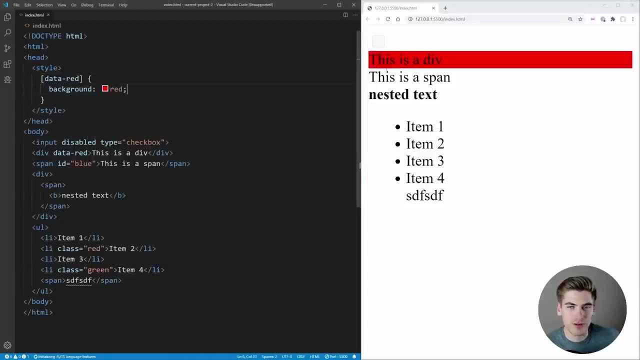 our div. now, in order to select elements based on data attributes, you put them inside of brackets and then we just type in our attribute: data red has a background of red and now you can see this div has a background red because it matches this data attribute of red. that's pretty self-explanatory. 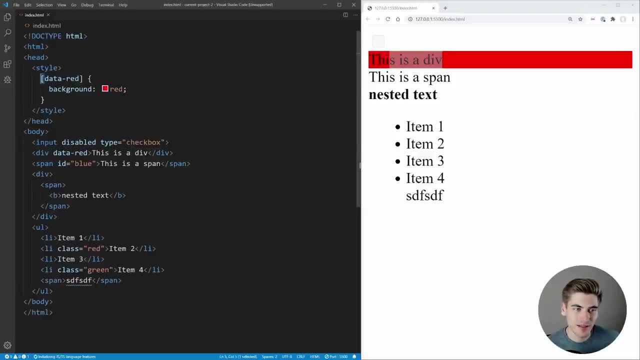 it's a lot like your class selector, except for here you just wrap it in brackets. what if you want to check for particular value? let's say we want to say data red is true. what if we want to check for that particular value? you just say equals and then inside of quotes you put your value. in our case, 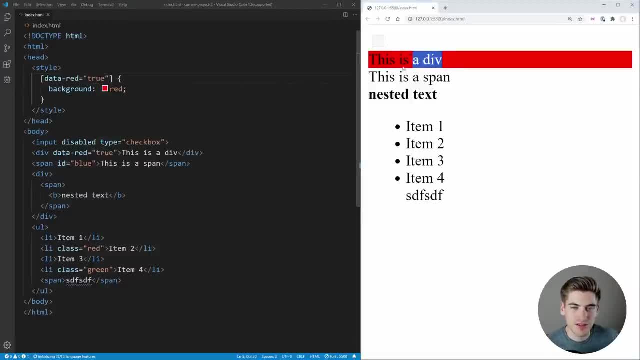 oops, true, now if we save, you can see this is still red because it matches that value. but if we change this to something else, like false, you can see that it is no longer matching this selector up here. but if we were to remove this equals section, it'll still match because it's just 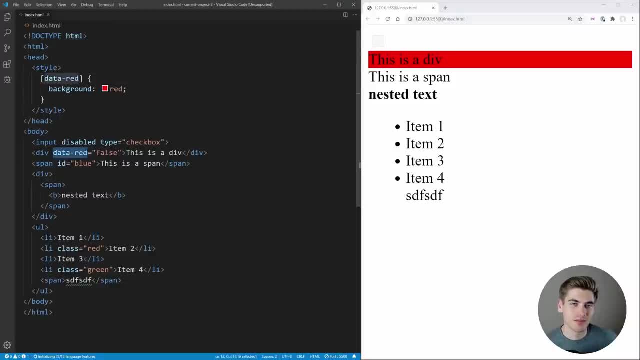 saying any class or any element that has that data attribute. it doesn't matter what the value is. i select it now, if we come over here, let's just change this to one, two, three and there's a few other ways that we can compare for values of our data attribute as opposed to just equals, because 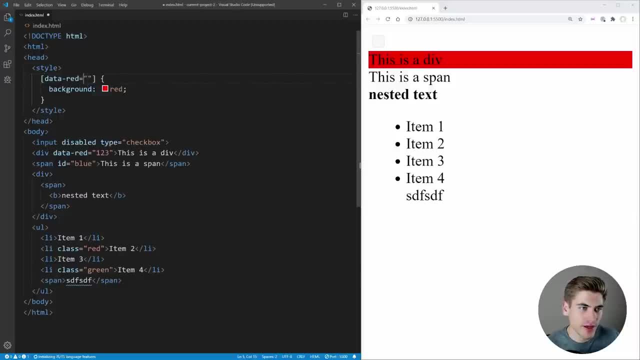 equals is saying exact match. what if we want to do a partial match? for example, if we wanted to say: i want the beginning of this to start with a one two, and you can see our color is red and that's because beginning of data at red begins with one, two. that's what this caret symbol equals does.